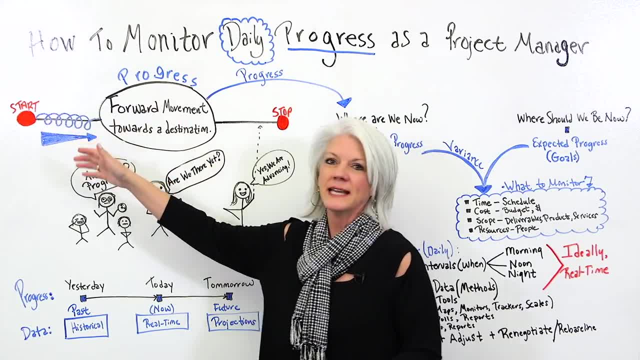 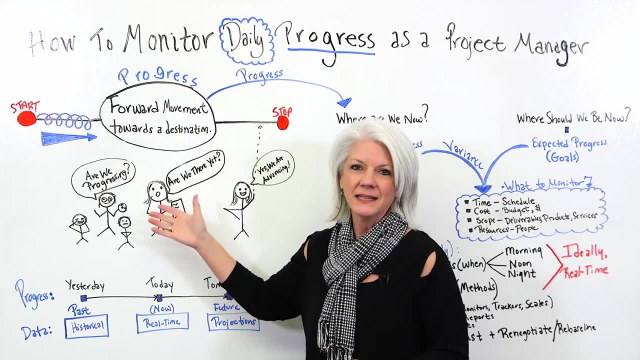 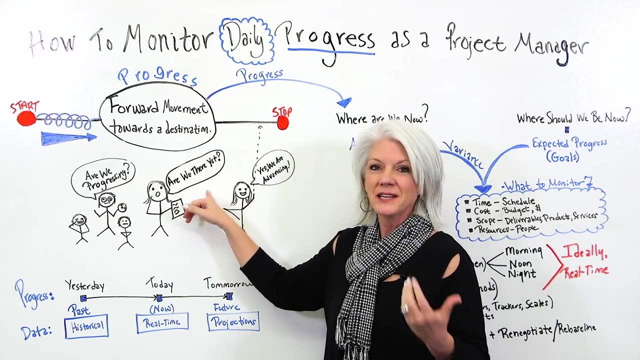 destination And on a project we have a start date and an end date, So we want to know when we started and when we stopped. So there are always people asking on the team, you know, are we progressing, Are we there yet? And sometimes people like to have an indication: yes, we are. 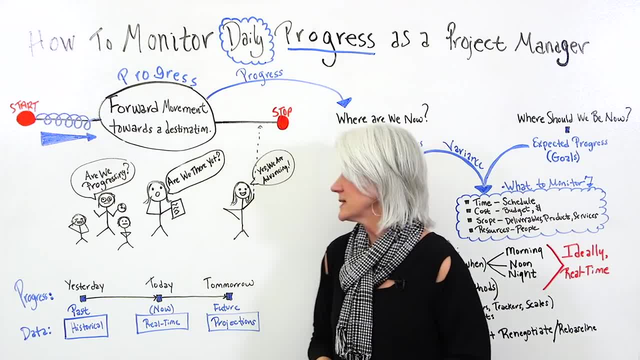 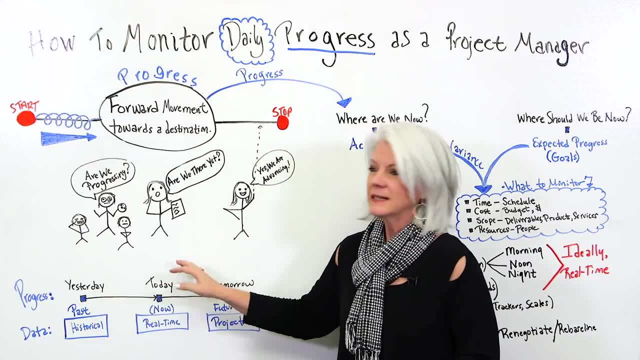 advancing, So that's good news. So when we talk about progress, we're looking at different time intervals. Sometimes we look at what did we do yesterday, So we're looking at the past. Sometimes we want to know what are we doing today, like right now, And then sometimes we're 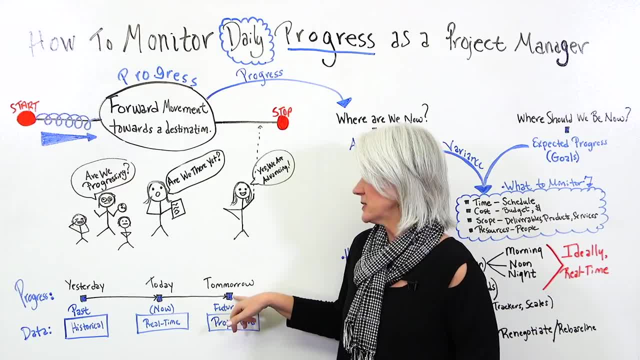 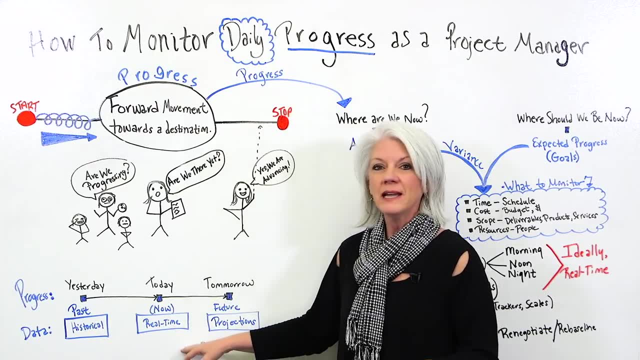 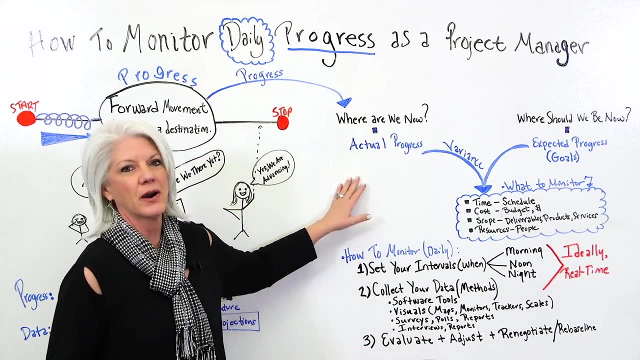 concerned about tomorrow. We want to know about future projections And when we look at this, all of this is some form of data. It could be historical, It could be real time Or it could again be projections. So now let's look at again. when we're looking at progress, we're looking at 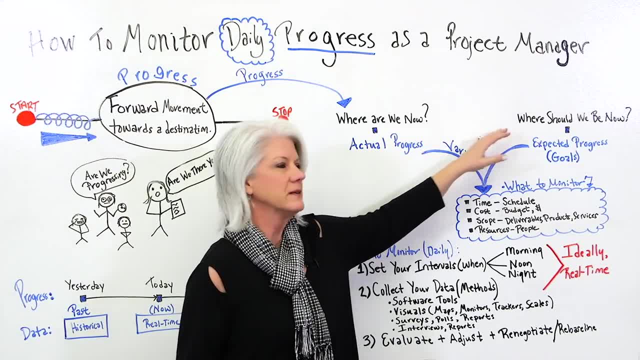 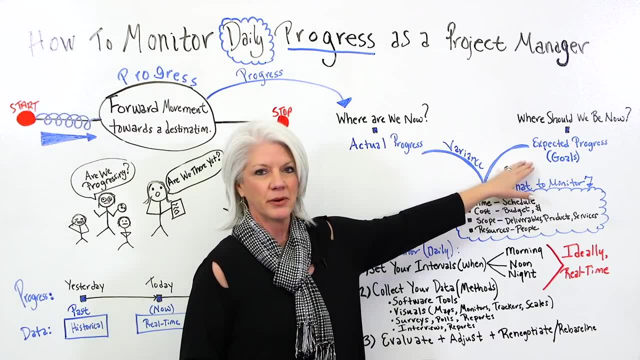 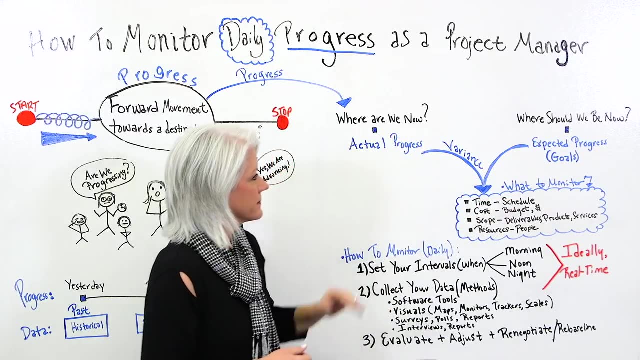 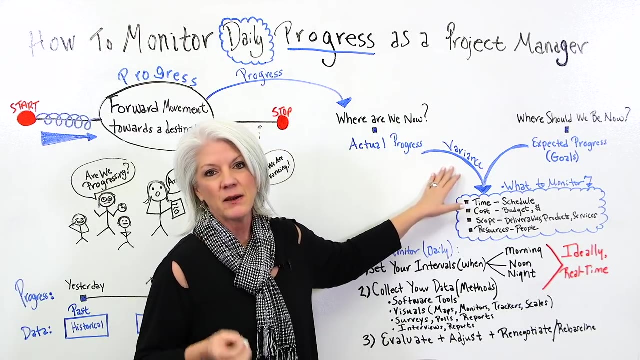 where are we now and where should we be? So if we look at where are we now, we're looking at the actual progress versus the expected progress, Our goals and many times, our contractual expectations. So when we look at the difference between these two, we're talking about some form of variance. And here are the things that we want to monitor. on a 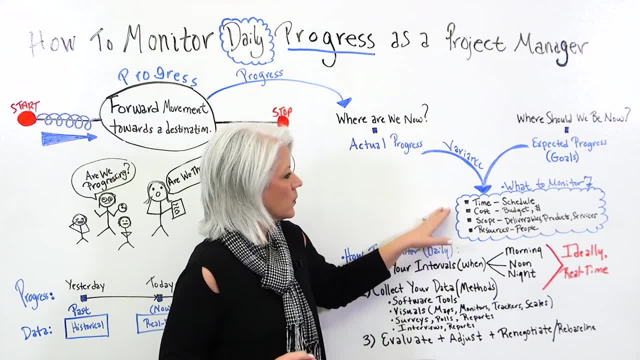 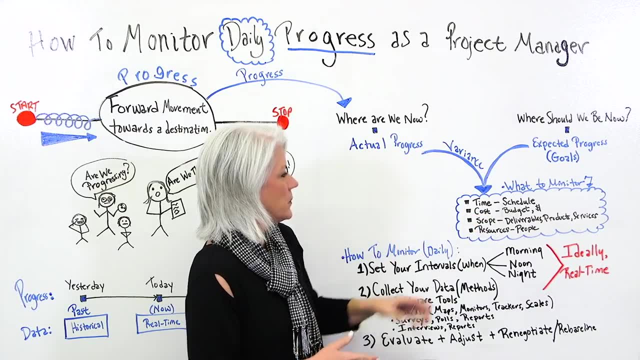 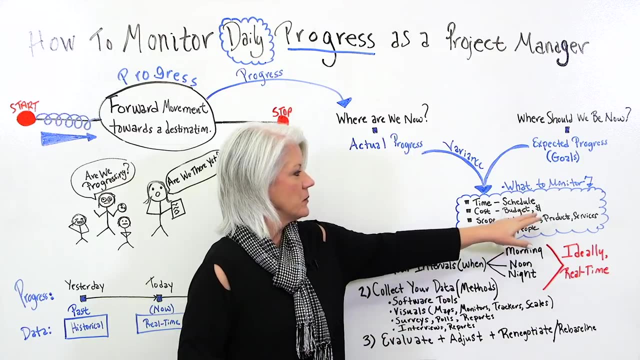 project. So we want to look at time. Where are we in relation to the schedule? Are we ahead of schedule? Are we behind schedule? We also want to look at the cost, specifically our budget. Are we exceeding our budget? We want to know about the money. So we also want to look at scope, because scope- 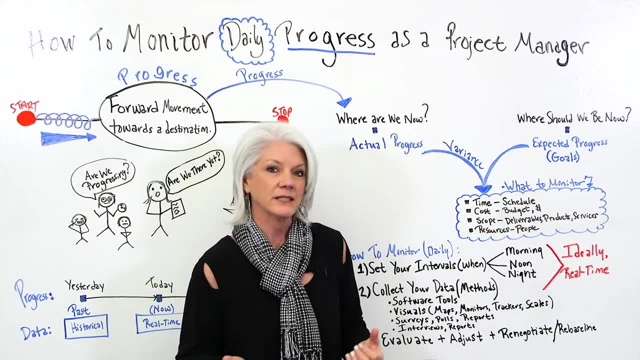 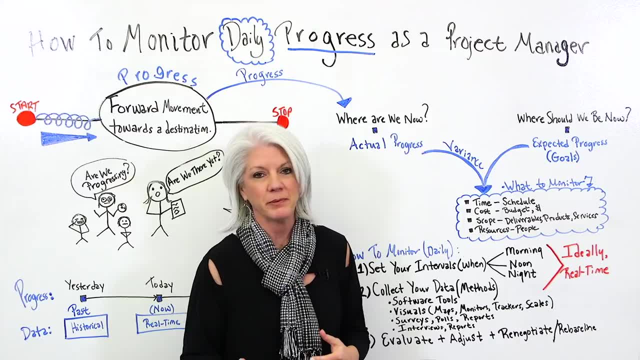 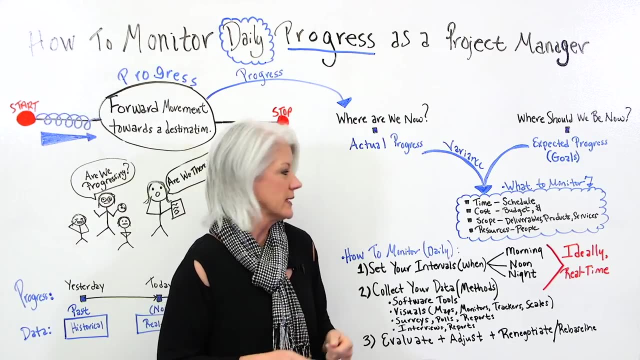 begins to be the deliverables we're producing, the products or maybe the services. And then we also want to look at people. Do we have enough people? Do we have too many people? How do we need to compensate? So let's look at how we monitor and, specifically, we want to look at daily. So, first of 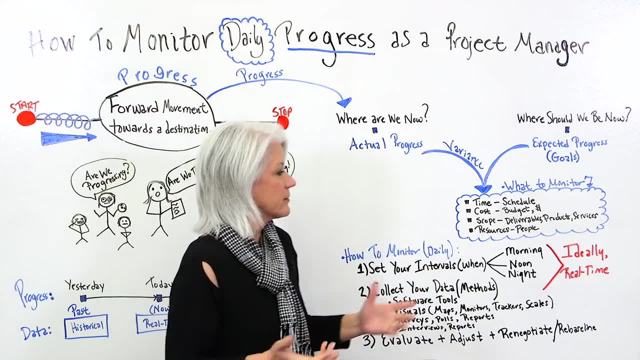 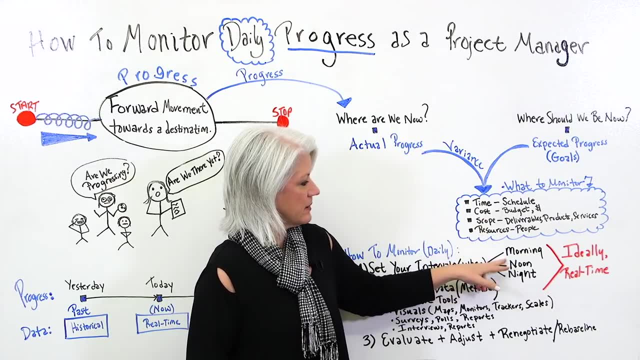 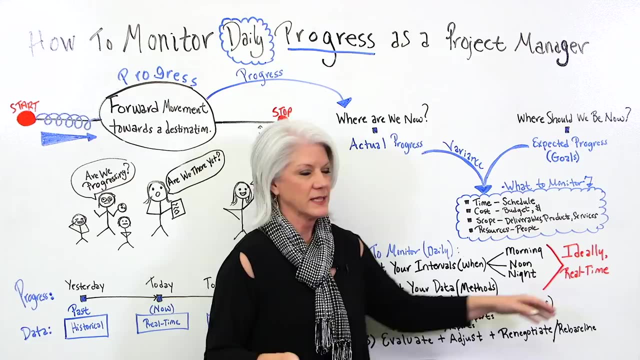 all. you set your intervals of when you want to monitor. For instance, if you're monitoring daily, you may want to look at specific reports or projections in the morning, maybe at noon or even at night, And ideally, on a project, you're looking at things real time.